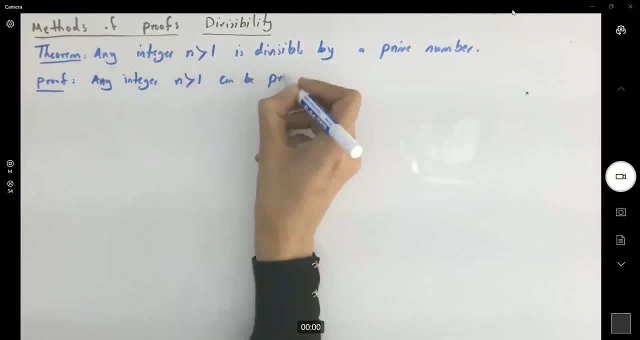 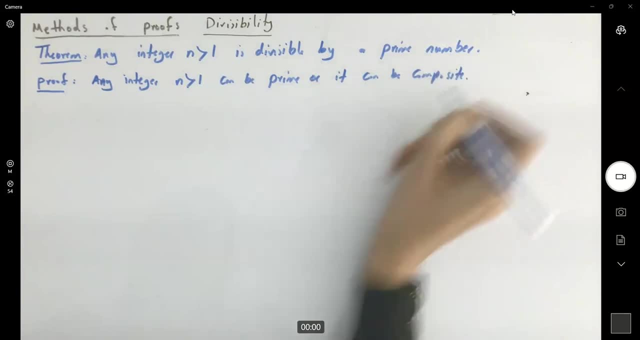 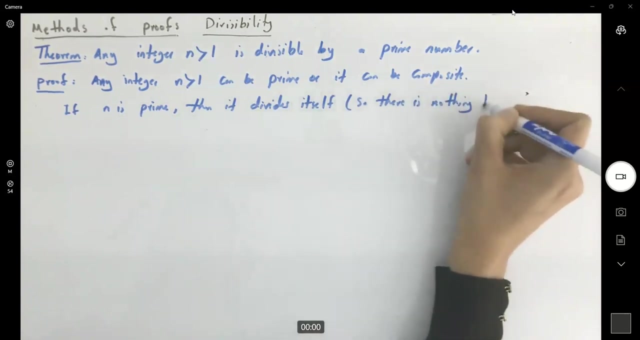 like n larger than one can be prime or it can be composite. So let us begin the proof. Any integer like n larger than one can be prime or it can be composite. So if it's prime, if n is prime, then it divides itself. So there is nothing to prove. 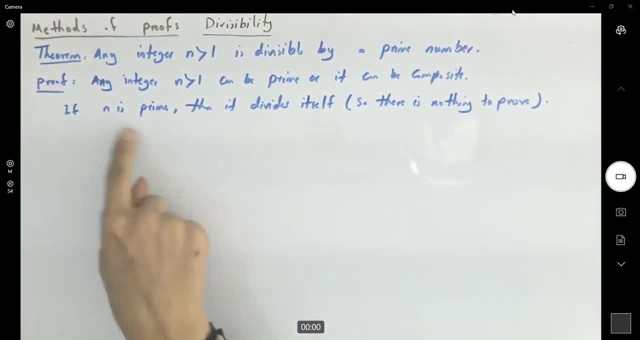 This is the very first scenario. If n is a prime number, then it divides itself. It's a factor of itself, So there is nothing to prove. However, if it's composite, you have the following scenarios: If n is composite, then by definition n can be written as the multiplication of two integers. 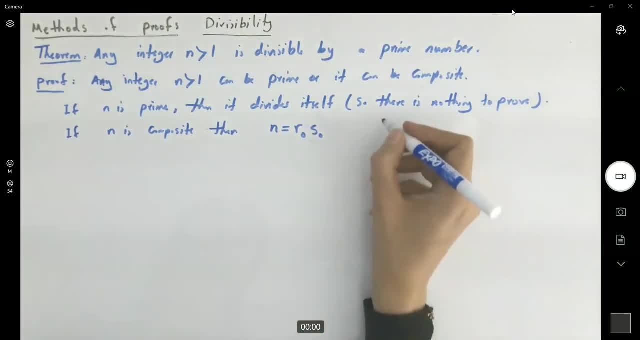 like r sub 0, s sub 0,, such that n is a prime number. If n is a prime number, then by definition n can be written as the multiplication of two integers like r sub 0, s sub 0,, such that r sub 0 is bounded between 1 and n and s sub 0 is bounded between 1 and n. 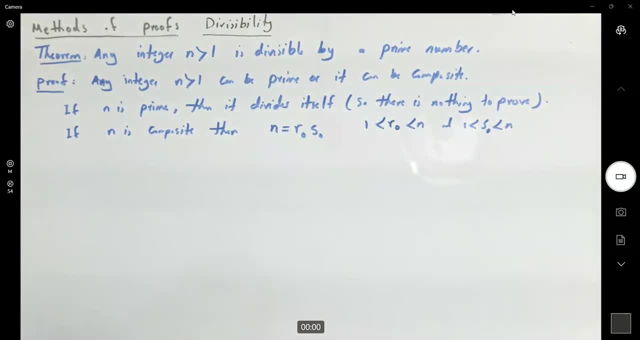 This is how we define a composite number. Okay, What's the scenario then? n is r sub 0 times s sub 0.. This means that r sub 0 times s sub 0.. This means that r sub 0 times s sub 0. 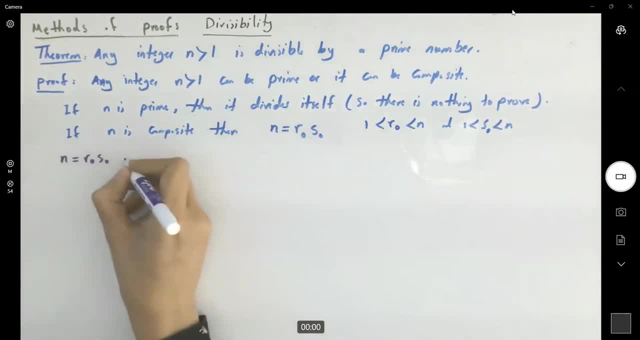 This means that r sub 0 times s sub 0.. n equals to r sub 0, s sub 0, means that r sub 0 divides n and also s sub 0 divides n. If one of them is prime, then we're done. 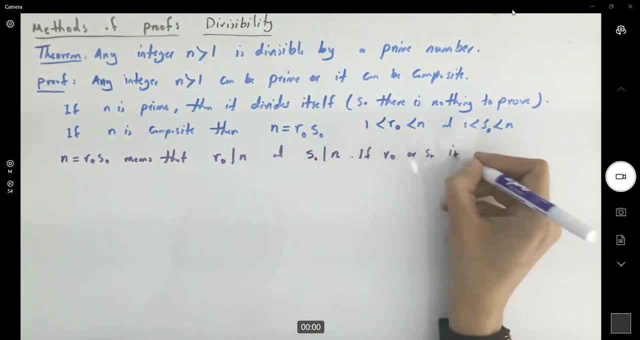 r sub 0 or s sub 0 is prime, then you're done. We try to show that any n is a prime number. Any integer is divisible by prime number, Then we are done. If not, if none of r sub 0 and s sub 0 are prime numbers, then we're done. 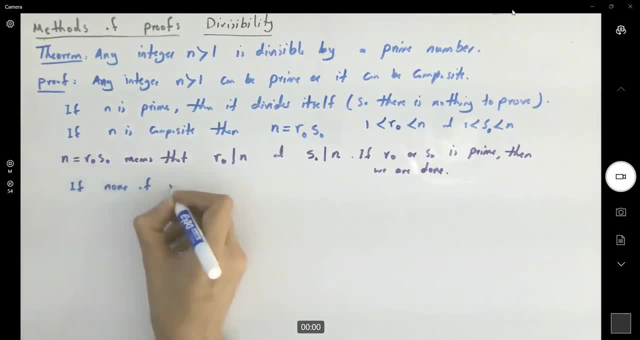 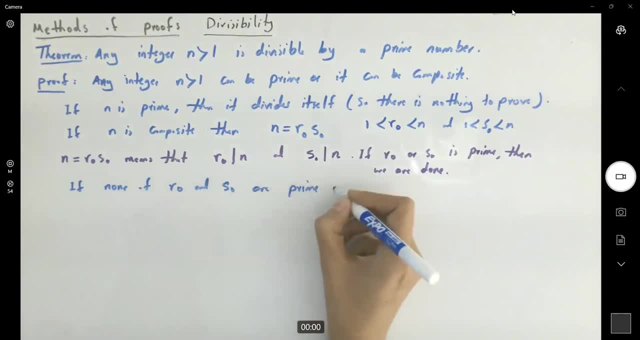 If none of r sub 0 and s sub 0 are prime numbers, then we're done. If none of r sub 0 and s sub 0 are prime numbers, then we're done. are prime numbers, then they are also composite. so what's the meaning of that? it means that 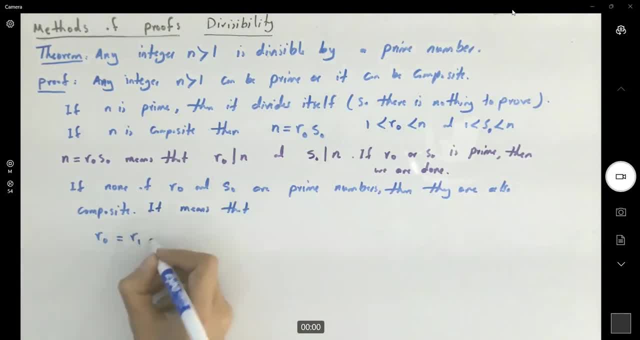 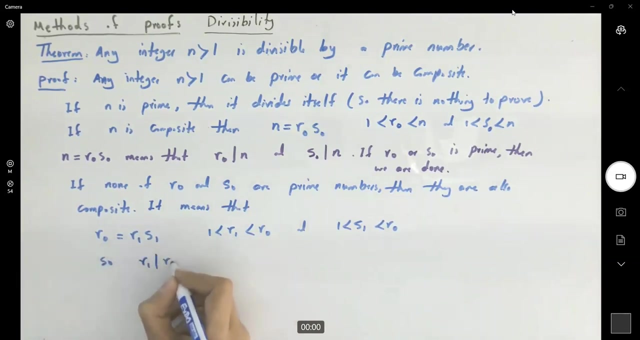 r sub 0 can be written as r sub 1, s sub 1, r sub 1 is bounded between 1 and r sub 0, and s sub 1 is bounded between 1 and r sub 0. okay, so what's the meaning of that? so r sub 1 divides r sub 0. 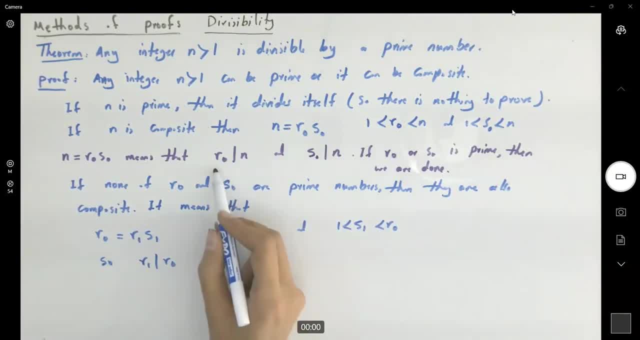 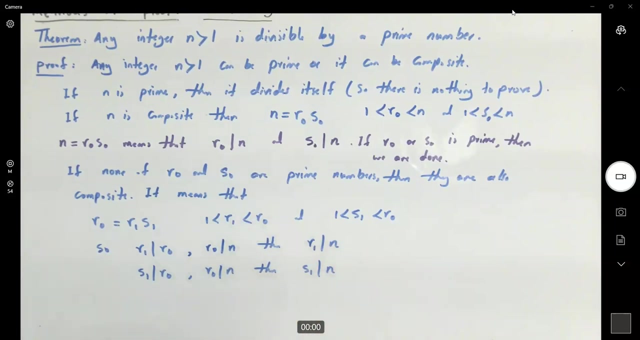 and by transitive property. since r sub 0 divides n, then r sub 1 divides n. s1 divides r sub 0. since r sub 0 divides n, then s1 divides n as well. again, if either r1, s1 are prime numbers, then we're done. we found a prime factor. 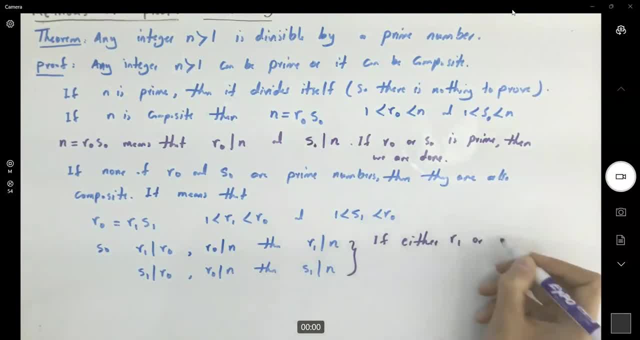 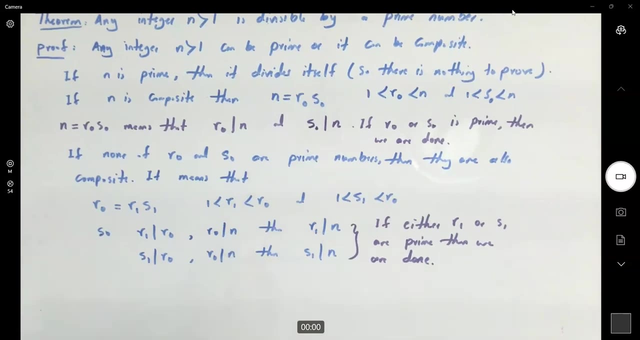 if either r1 or s1 are prime, then we are done. if not, we have to continue this process. none of r sub 1 or s sub 1 are prime, then we have to continue this process, this process until we can break them down into prime numbers.